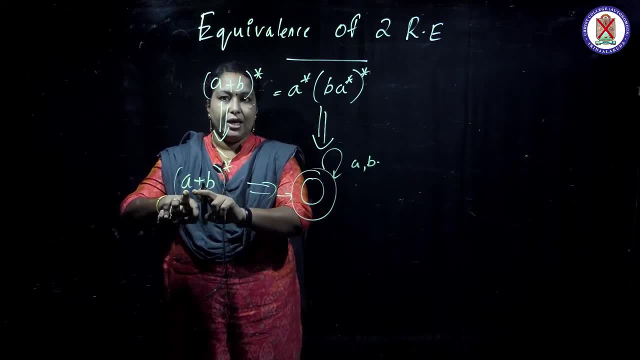 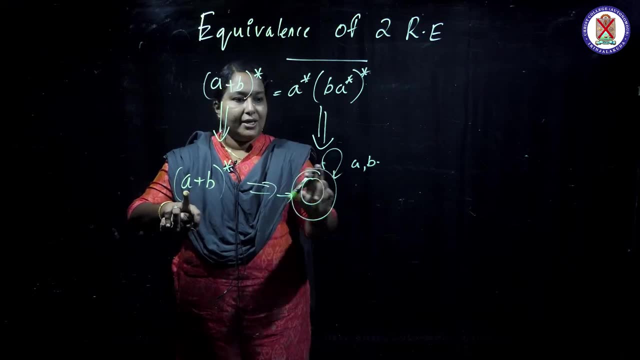 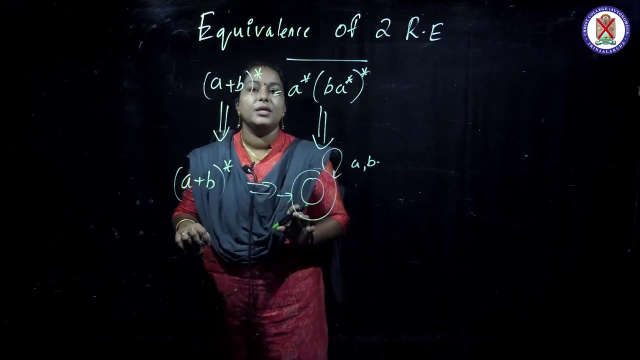 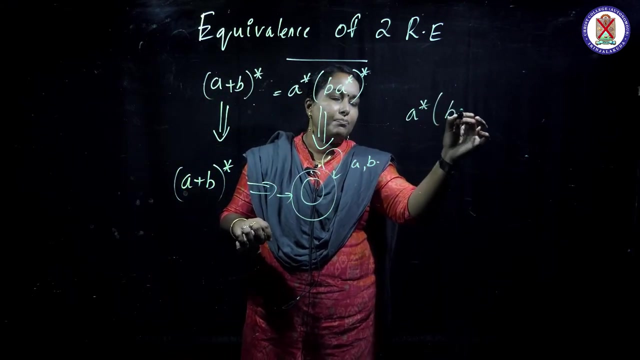 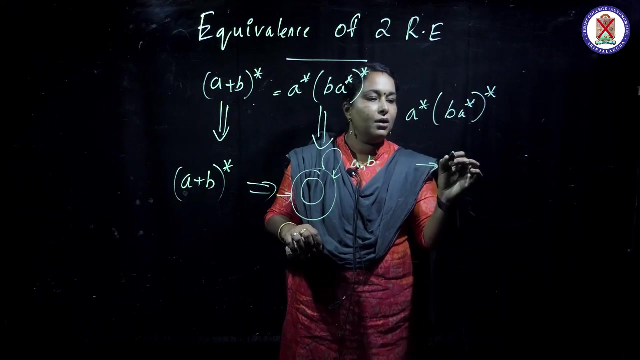 Why it is this: a plus b, whole star. Because b, a can be equal or b can be equal. It's star means zero or more combination, So whether a can occur or b can occur or both can be occurred, that is meant by the stars. So the DFA must like will be drawn like this: Next we have to draw the DFA for a star, b star, whole star. Okay, so I am drawing the DFA here. 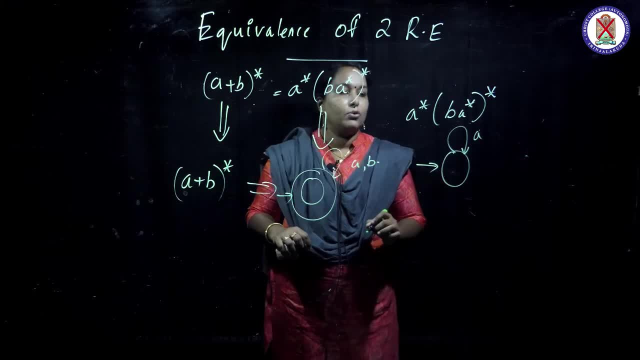 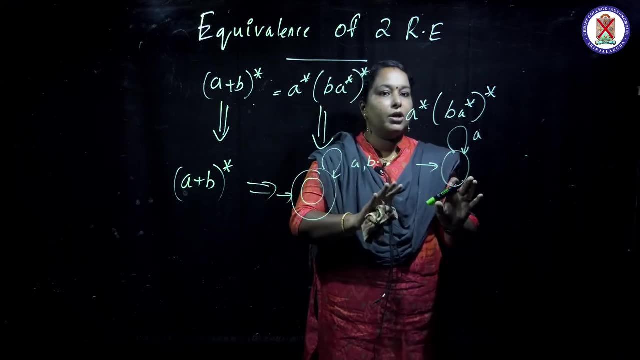 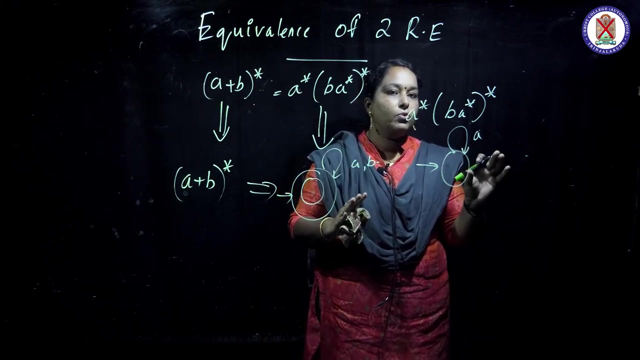 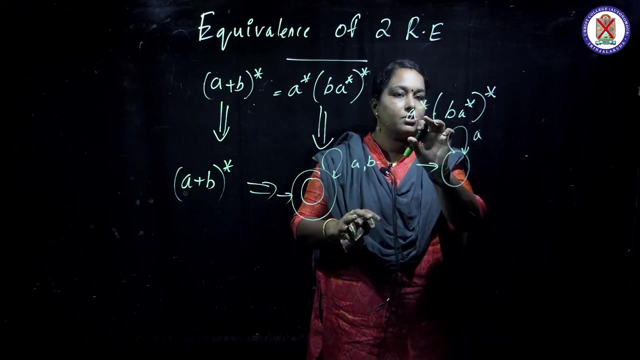 a star. a star means what a can occur or not. it's looped. star means zero or more combination, So it is been looped now. now, I am not drawing the minimized DFA. you must have in your mind the minimized DFA. but look at here we can follow the method so that you can easily minimize the DFA without going into the errors. Okay, so a star. I am drawing a single circle for the. a star means zero or more combination, So it is been looped now. now, I am not drawing the minimized DFA. you must have in your mind the minimized DFA. but look at here we can follow the method so that you can easily minimize the DFA without going into the errors. Okay, so a star. I am drawing a single circle for the. a star means zero or more combination, So it is been looped now. now, I am not drawing the minimized DFA. you must have in your mind the minimized DFA. but look at here we can follow the method so that you can easily minimize the DFA without going into the errors, Okay. 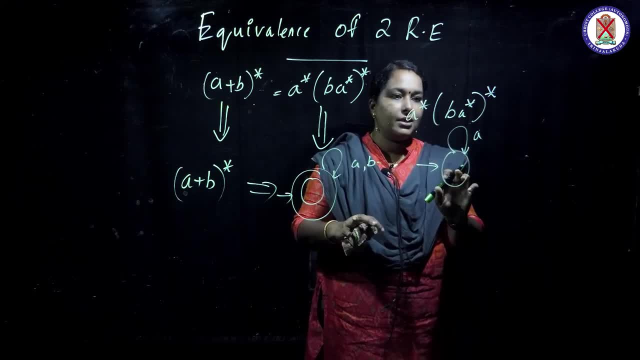 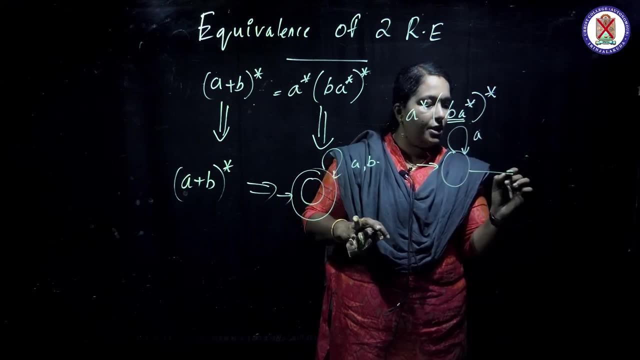 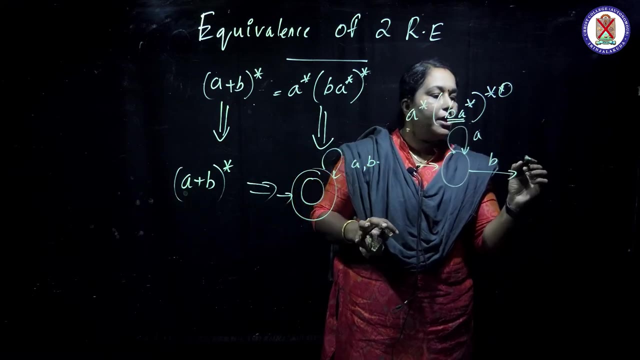 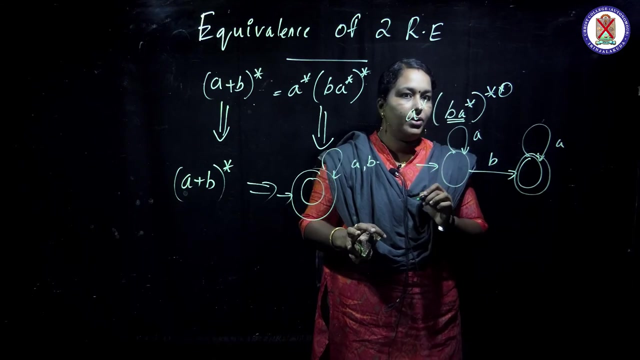 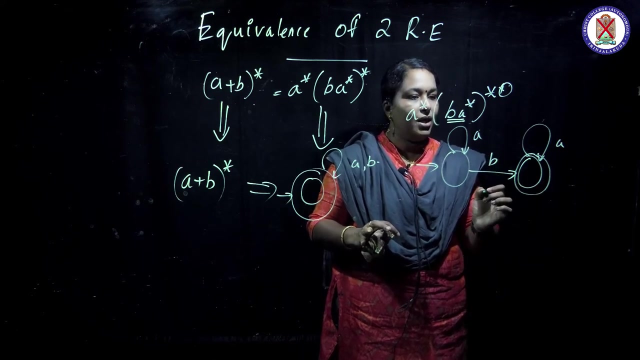 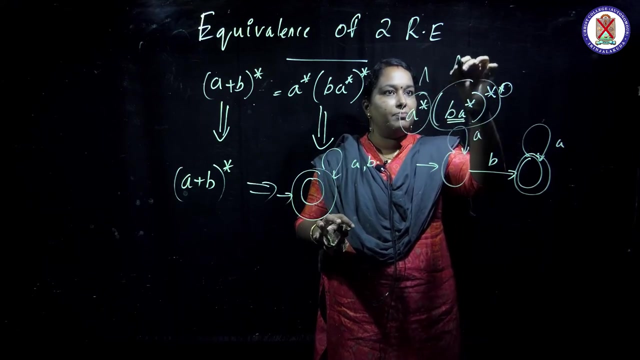 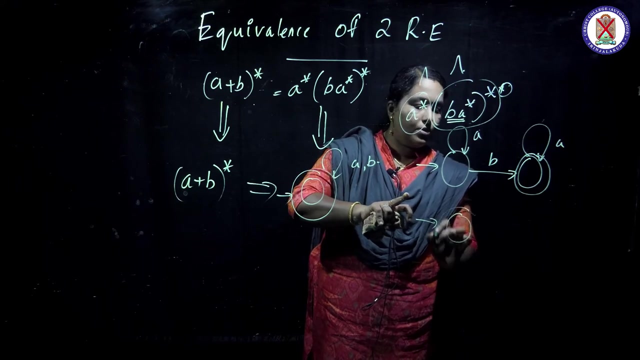 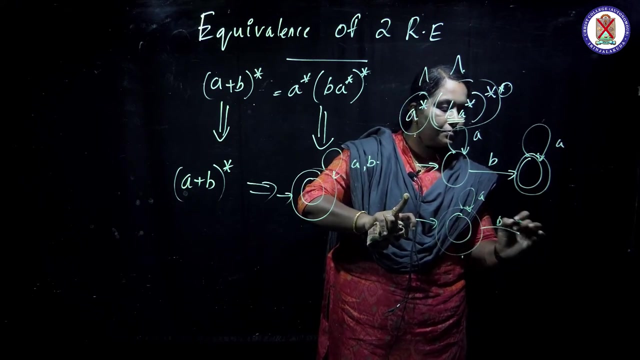 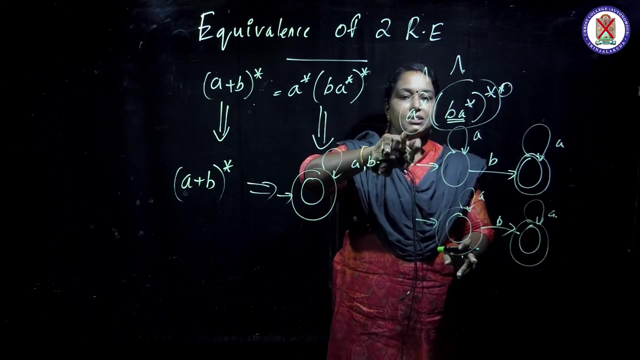